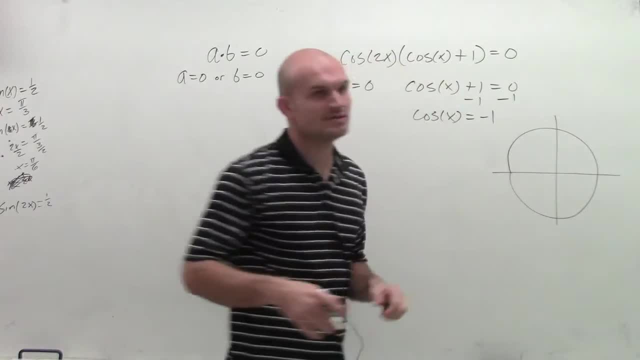 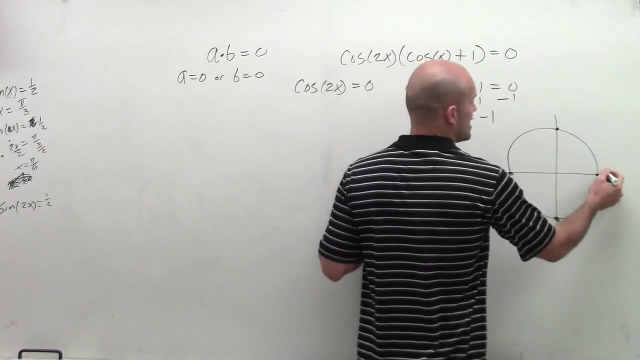 OK, so we go and drop our unit circle And remember the cosine represents your x-coordinate right. So we have four main intercepts on our unit circle. We have 1 comma 0,, 0 comma 1, negative, 1 comma 0, and 0. 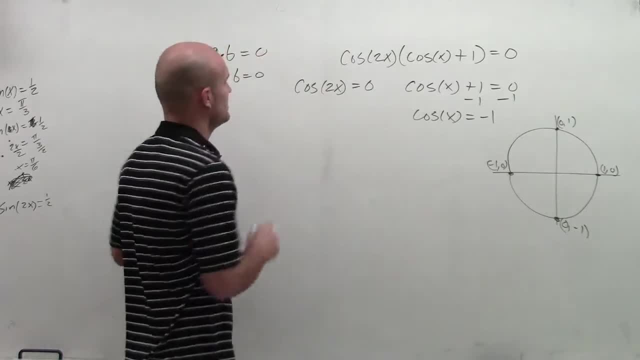 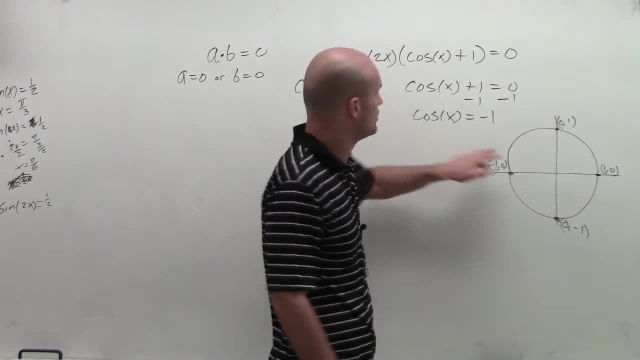 comma negative 1.. So in the first one we say: when is cosine equal to 0?? So that means: when is my x value equal to 0?? Well, we have two solutions. right, We have, x is going to equal or, I'm sorry, our cosine value is. 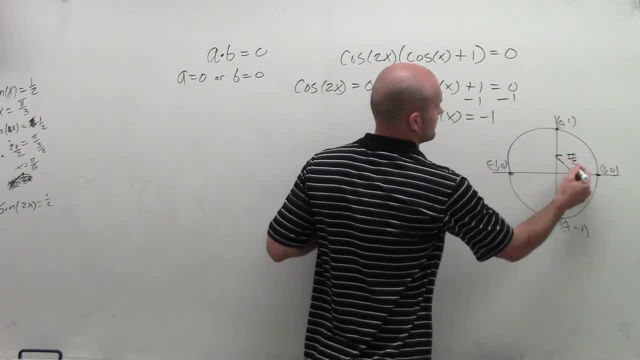 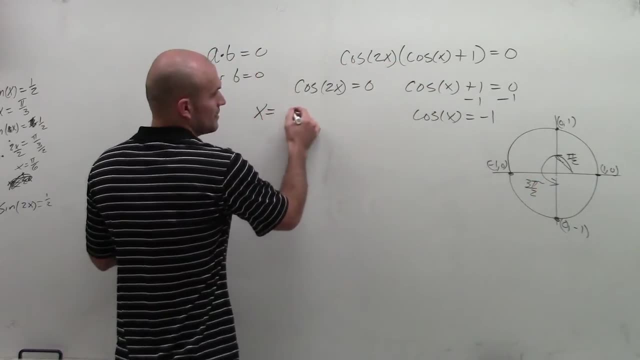 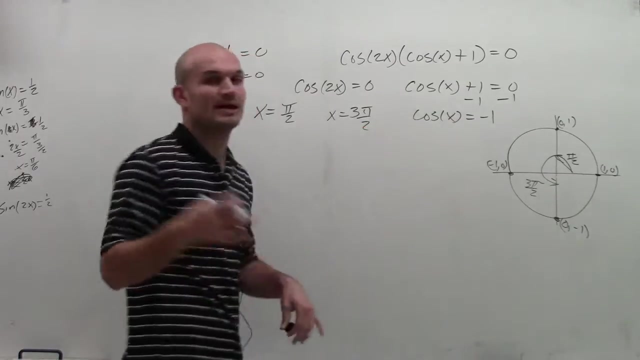 equal to 0 at pi halves and 3 pi halves. So therefore I can just simply write x equals pi halves and then x equals 3 pi halves, And I'll show you a different way to kind of write this up in a second. 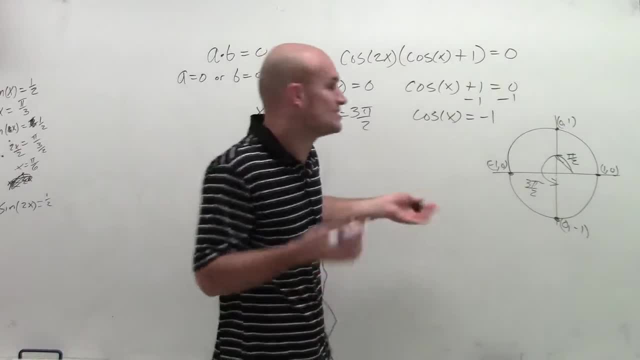 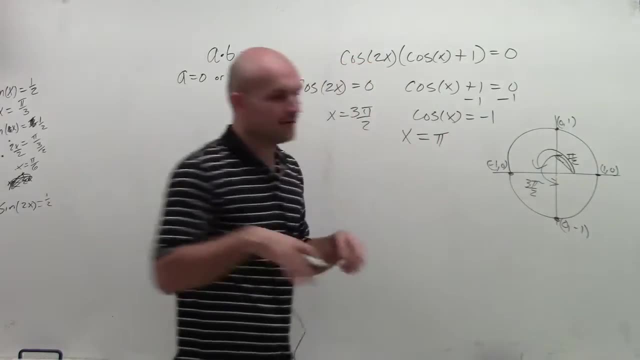 Then let's go and look at when is cosine equal to negative 1.. Well, the cosine value is only equal to negative 1 at one value, and that is that when x- equals halfway around circle is equal to pi. Now remember, when dealing with solving an equation, 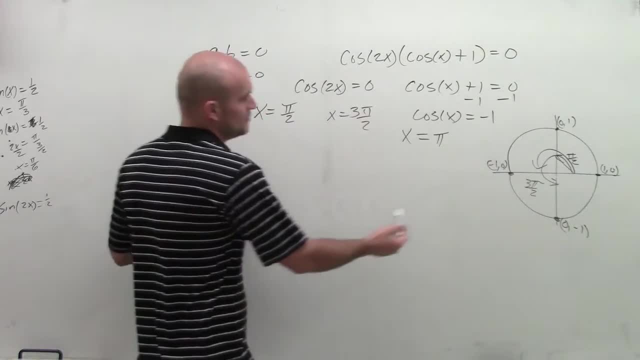 we need to include all the values that are going to make it true. So if you look at this- if I know pi halves is true- that means if I add pi to it, I'm going to get to 3 pi over 2, which is true. 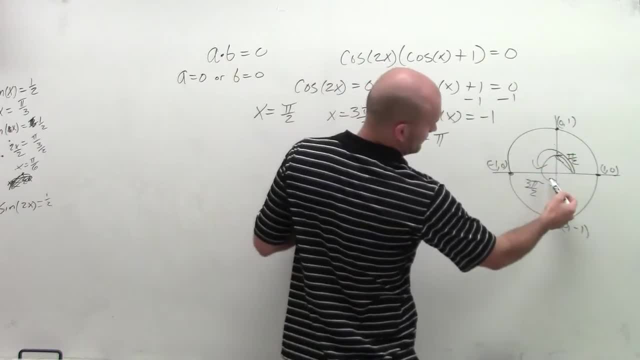 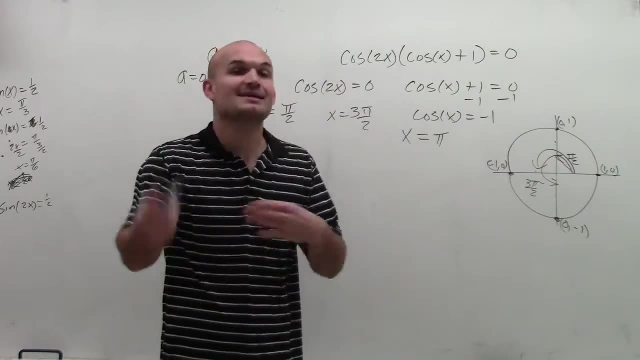 Then if I added a pi again, I'm going to get to pi 3, pi 4, pi, 5, pi halves, And then I could add it again And I get 7 pi halves. and I can continually keep on doing this. 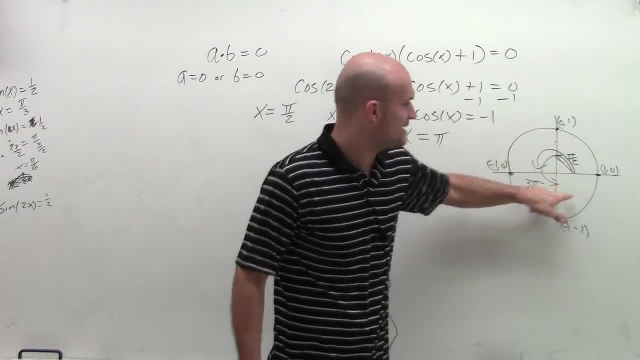 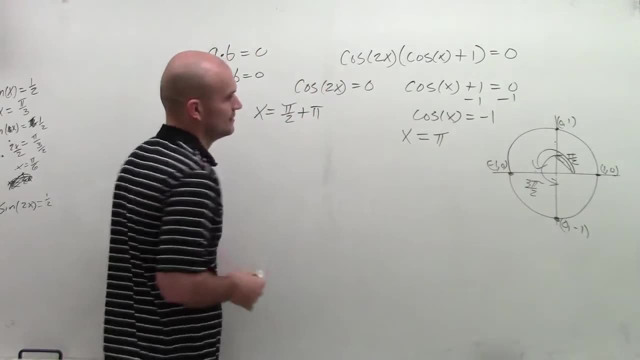 Now you notice, I could keep on adding 2 pi for this problem and I could keep on adding 2 pi to this angle. But why keep on doing that when all I simply need to do is, for one angle, just add pi, right. 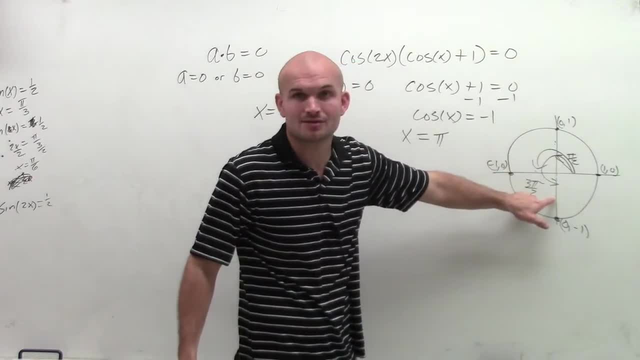 If I had pi halves and then I add the angle pi, I'm going to get to our next solution. If I add pi again, I'm going to get to another solution: Add pi again, so I can keep on adding pi. 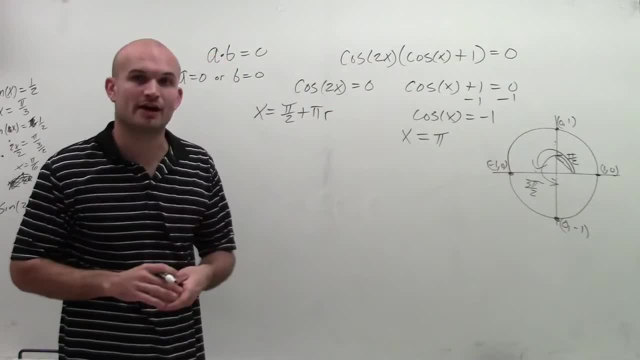 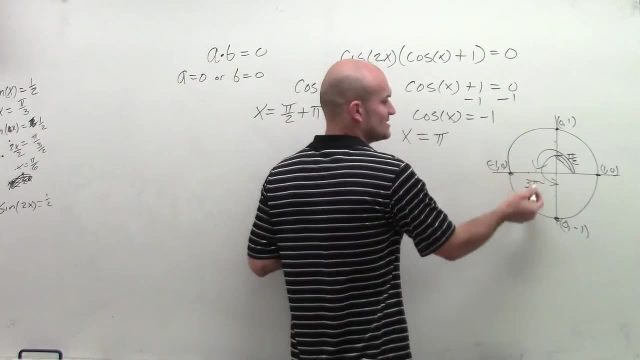 So, therefore, how many times can I add pi? We don't know, so we're going to leave it with the variable r. Now I look at x. x equals pi, But this is the only solution where my cosine of x equals negative 1.. 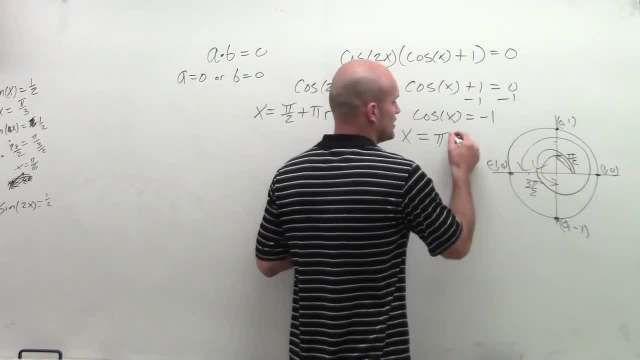 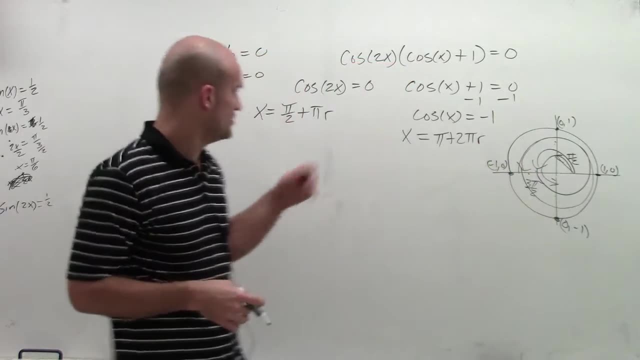 So to keep on finding more solutions, I'm going to need to add a full revolution, which is going to be 2 pi, And then I can keep on doing that r many times. So therefore I have x equals, pi, halves plus. I'm sorry. 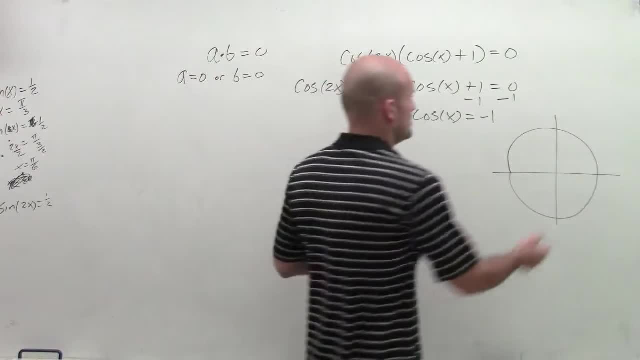 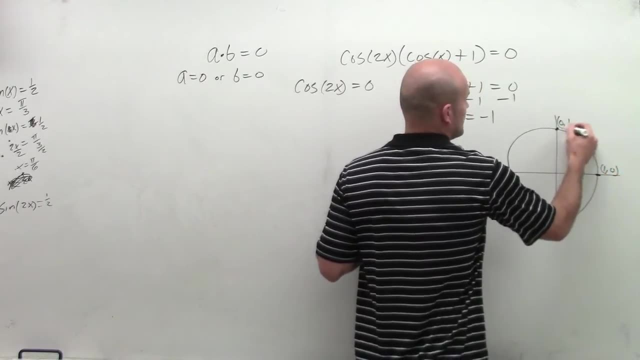 And remember the cosine represents your x-coordinate. So we have four main intercepts on our unit circle. We have 1 comma 0, 0 comma 1, negative 1 comma 0, and 0 comma negative 1.. 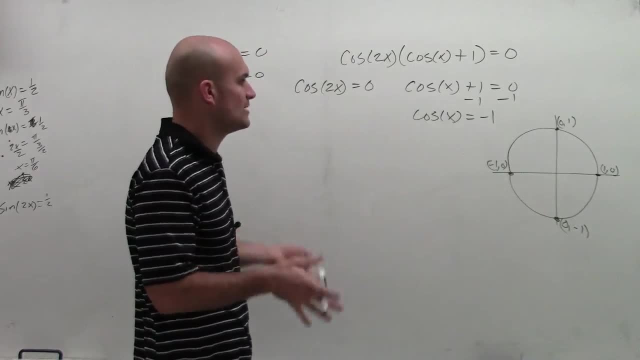 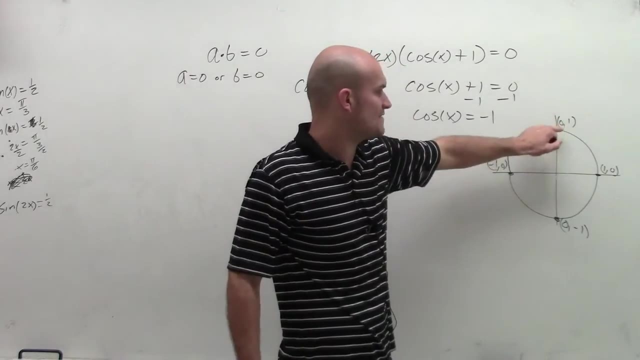 So in the first one we say: when is cosine equal to 0?? So that means, when is my x value equal to 0?? Well, we have two solutions, right, We have: x is going to equal or, I'm sorry, our cosine value is. 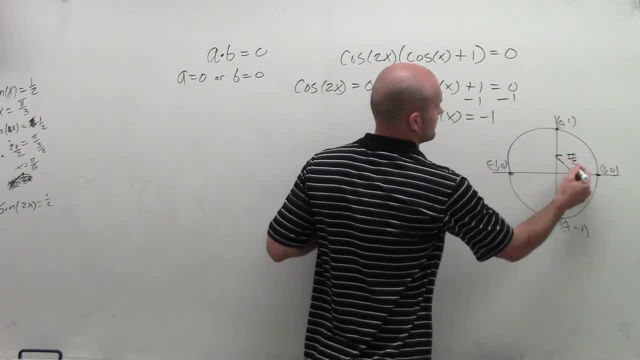 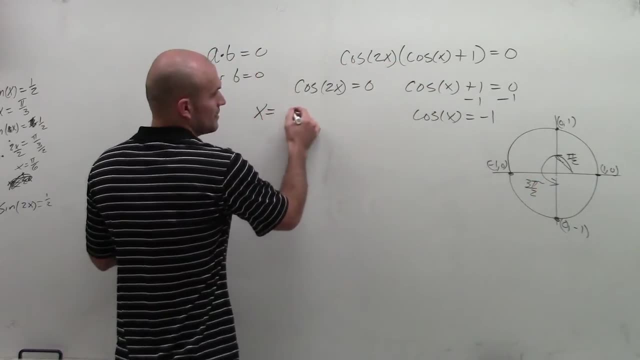 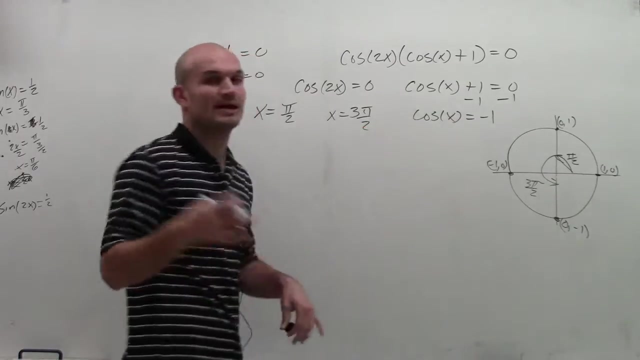 equal to 0 at pi halves and 3 pi halves. So therefore I can just simply write x equals pi halves and then x equals 3 pi halves, And I'll show you a different way to kind of write this up in a second. 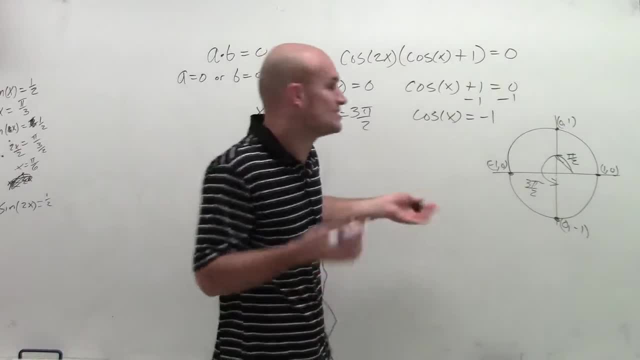 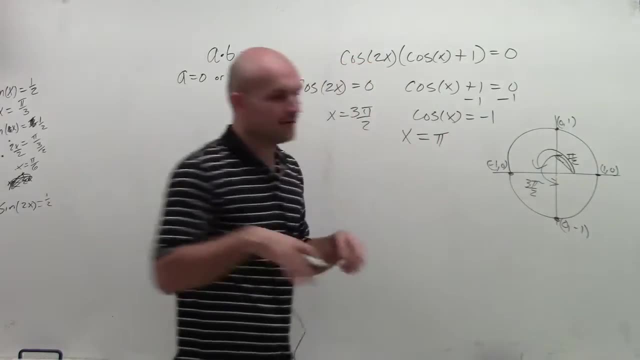 Then let's go and look at when is cosine equal to negative 1.. Well, the cosine value is only equal to negative 1 at one value, and that is that when x- equals halfway around circle is equal to pi. Now remember, when dealing with solving an equation, 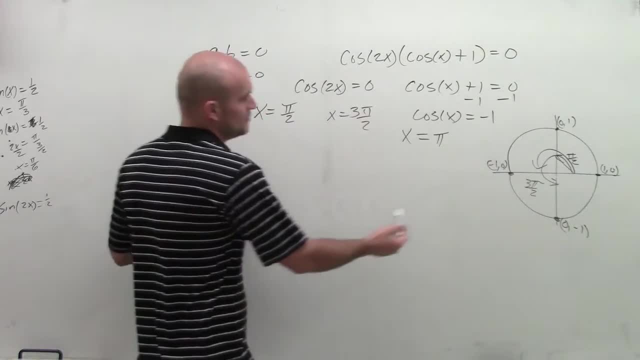 we need to include all the values that are going to make it true. So if you look at this- if I know pi halves is true- that means if I add pi to it, I'm going to get to 3 pi over 2, which is true. 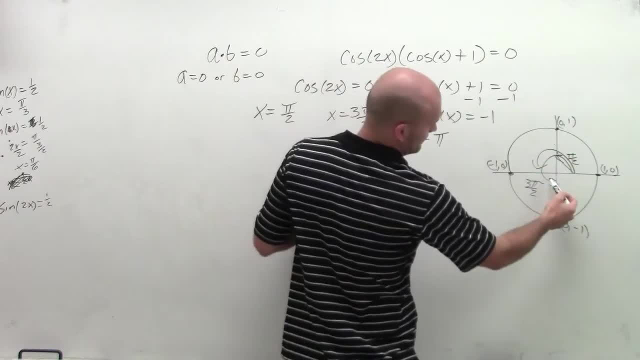 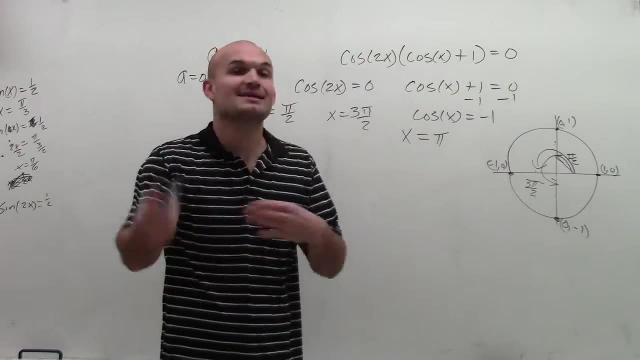 Then if I added a pi again, I'm going to get to pi, 3, pi, 4, pi, 5 pi halves, and then I can add again and I get 7 pi halves, and I can continually keep on doing this. Now you notice, I can keep on adding 2 pi for this problem. 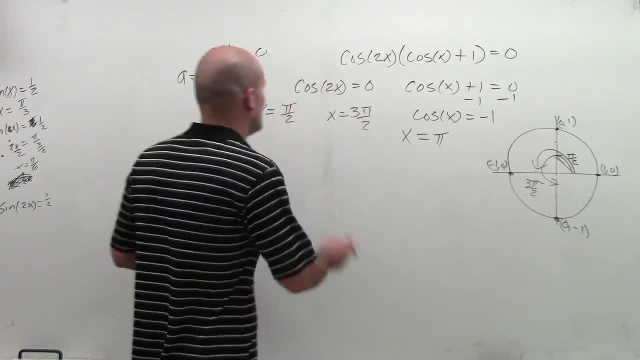 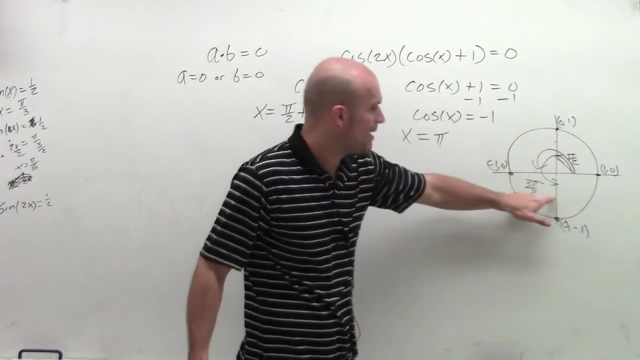 and I can keep on adding 2 pi to this angle. But why keep on doing that when all I simply need to do is, for one angle, just add pi, right, If I had pi halves? and then I add the angle: pi. 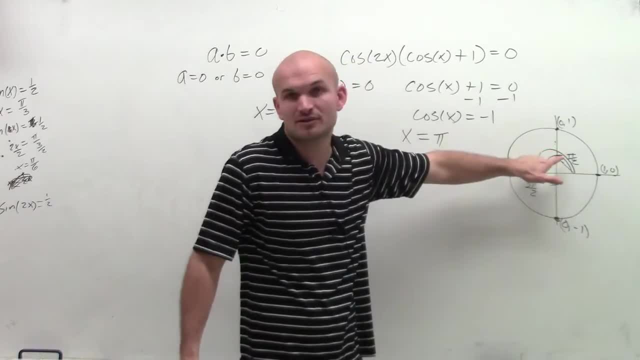 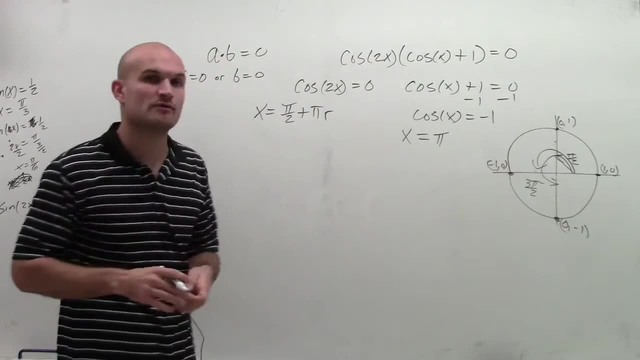 I'm going to get to our next solution If I add pi again. I'm going to get to another solution: Add pi again, so I can keep on adding pi. So therefore, how many times can I add pi? We don't know, so we're going to leave it with the variable r. 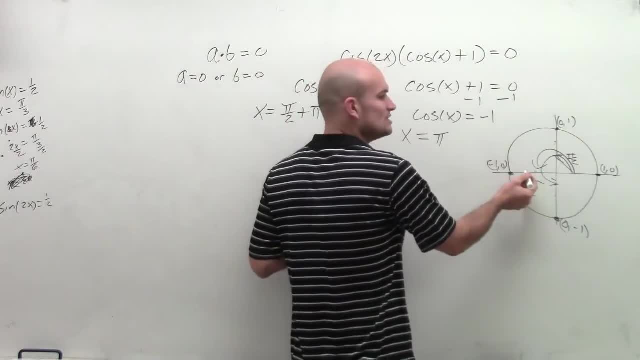 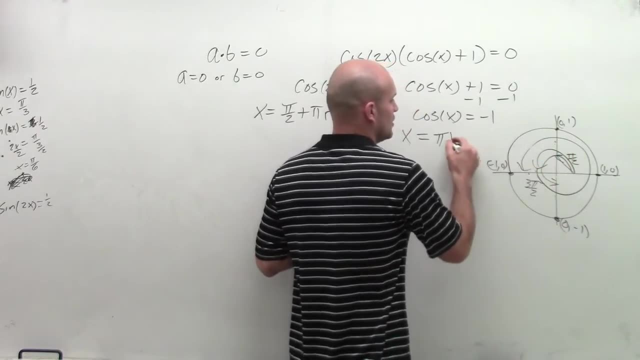 Now I look at x. x equals pi, but this is the only solution where my cosine of x equals negative 1.. So to keep on finding more solutions, I'm going to need to add a full revolution, which is going to be 2 pi. 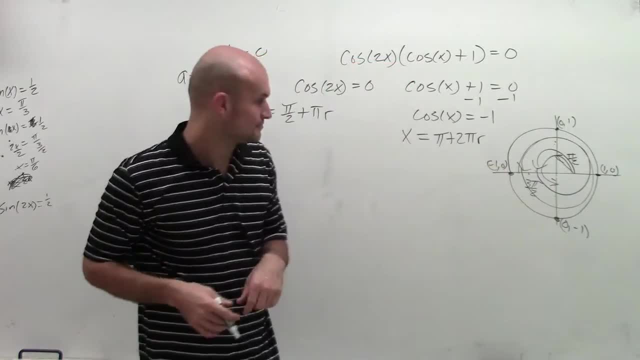 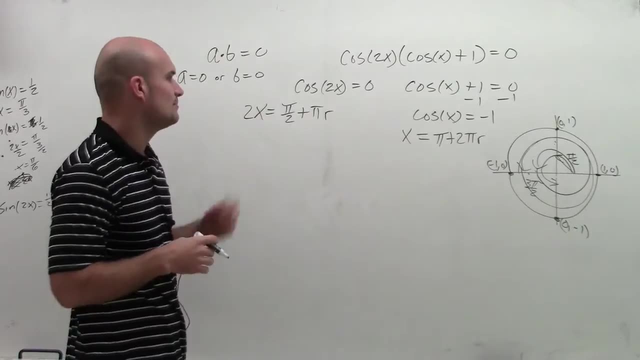 And then I can keep on doing that r many times. So therefore I have x equals pi halves plus- I'm sorry, that's 2x equals pi halves plus pi times r, and x equals pi plus 2 pi r. Now to finish up my multiple angle. 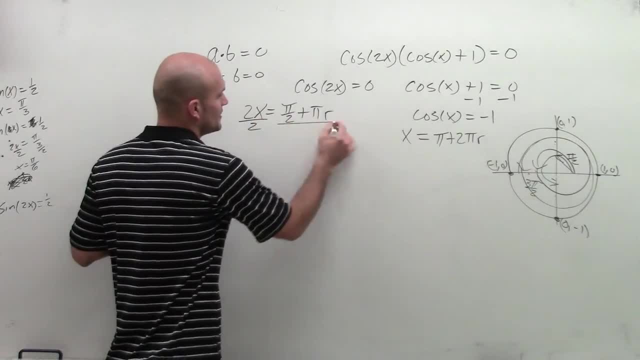 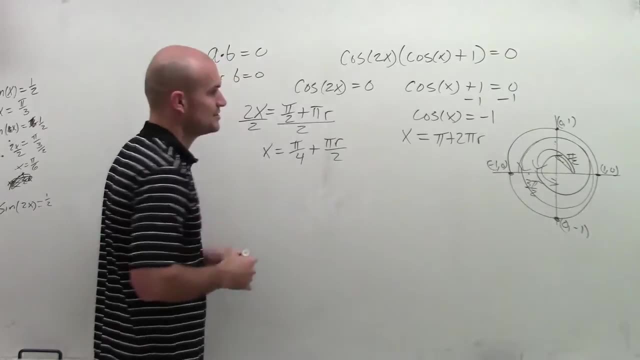 we need to solve for x, right? So therefore, what I'm simply going to do is just divide by 2 here, And I get x equals pi divided by 4, plus pi r divided by 2.. And over here I just have x equals pi plus 2 pi times r. 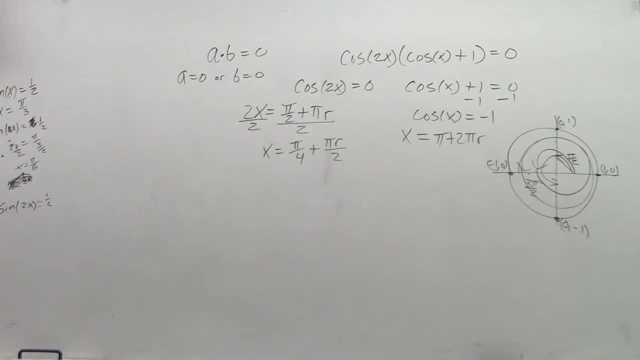 There you go, ladies and gentlemen. Hope you enjoyed Thanks. 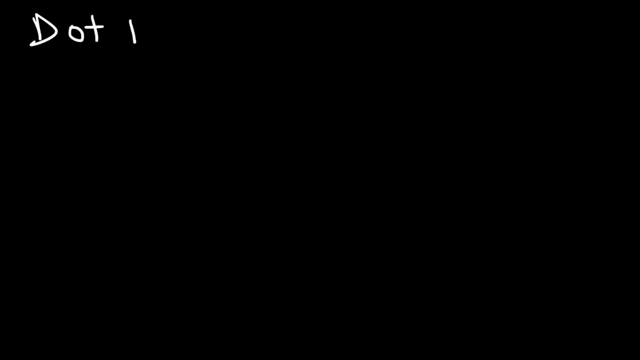 In this lesson, we're going to focus on the dot product, which is one of two ways to multiply two vectors together. 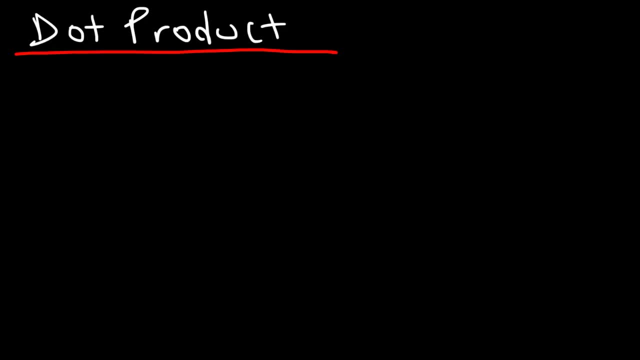 The difference between the dot product and the cross product, which is the other way, is that the dot product, it gives you a scalar quantity after multiplying two vectors. 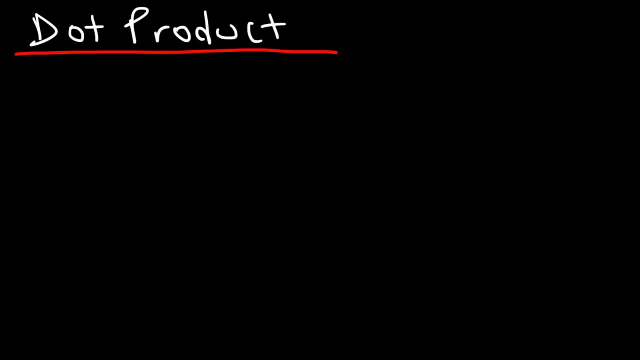 The result of the cross product, on the other hand, is a vector quantity. 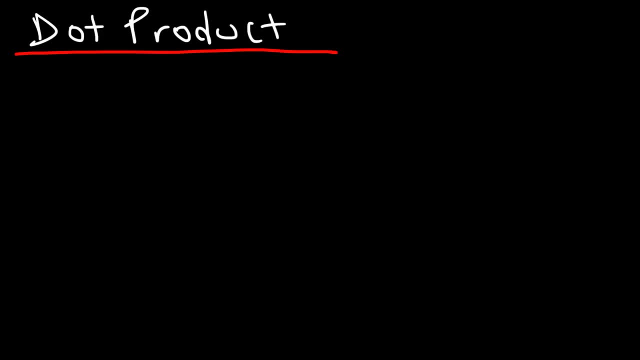 So let's work out an example. But first, let me give you the formula. So let's say if we have vector A with its x component and its y component, and vector B with its x and y components. 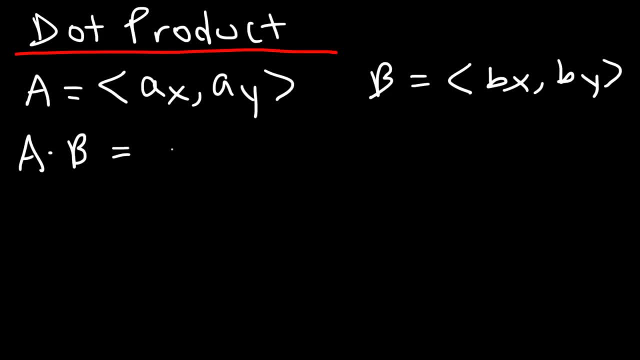 The dot product of A and B is simply the product of the x components plus the product of the y components. So it's Ax times Bx plus... Ay times By. 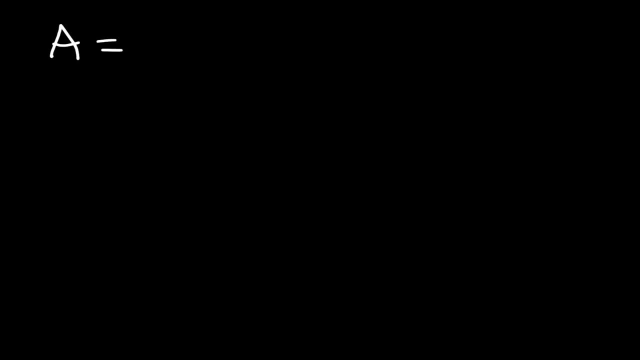 So let's try an example. So let's say vector A is 2,3 and B is 5,-4. 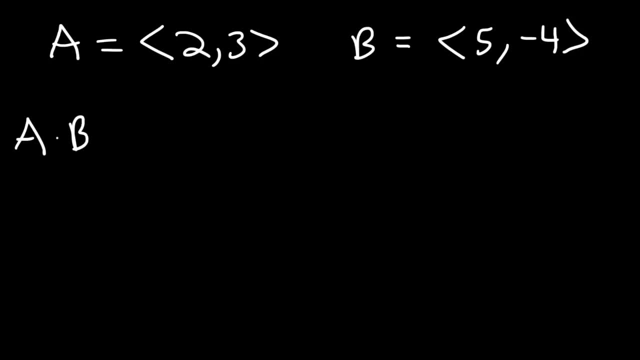 Go ahead and calculate the dot product of these two vectors. Feel free to pause the video if you want to. 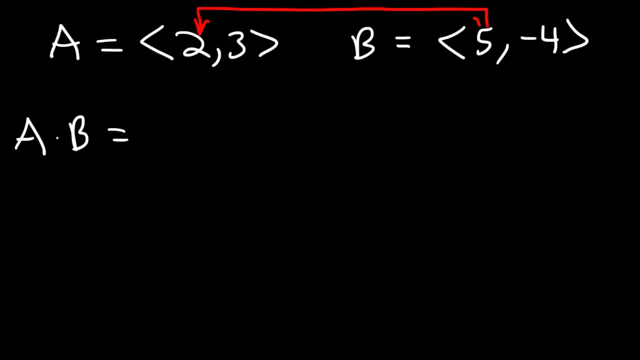 So the first thing we're going to do is multiply... ...these components. So we have 2 times 5. And then we're going to multiply the y components. So this is going to be 3 times negative 4.